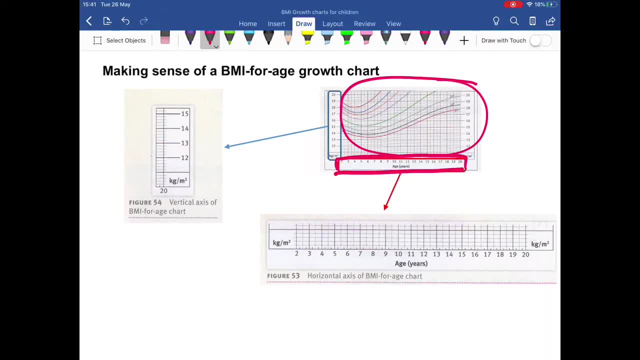 bottom. here we have the ages, So this ranges from two years to 20 years At the clinic. so if a child is younger than two years, there's another special growth chart that the clinic sisters use and that gets tracked more often than every year. 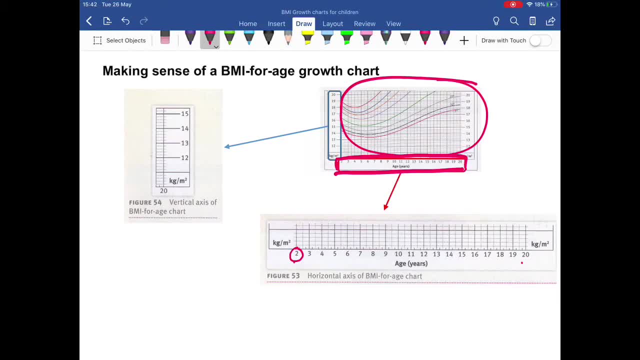 And in fact, every week when babies are just born, and then monthly, and then so the time stretches By 20, we should have reached our maximum growth spurt. Okay, so that's the age in years. And then at the side we have the vertical axis. 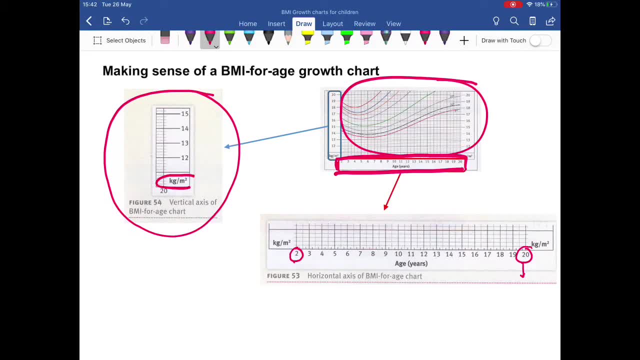 which shows the BMI. Now, if you can remember, BMI was measured in kilograms per meter squared And depending on what your BMI is, that would determine your weight status And from the weight status, the doctor can tell you whether you are eating. 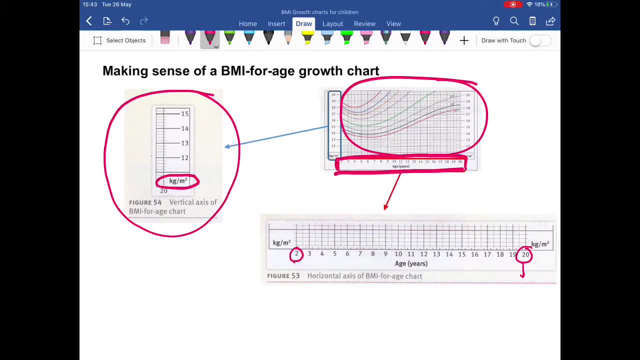 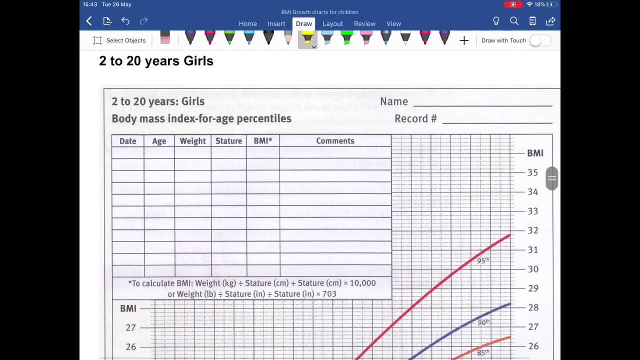 properly or you're developing properly. So let's go and have a look at the growth chart. Well, you will see. obviously there are different ones for girls than there are for from for boys, because we develop differently to what the boys do. 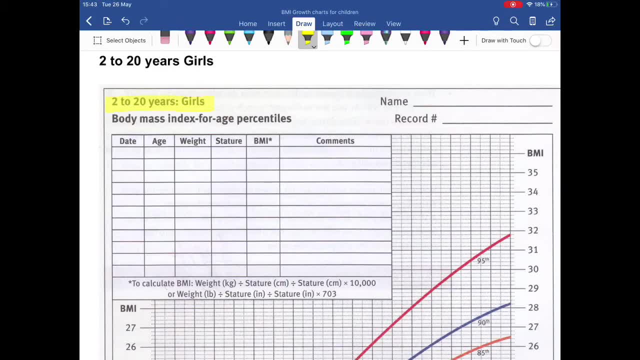 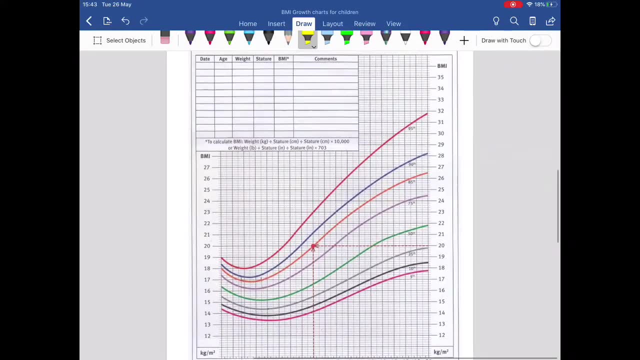 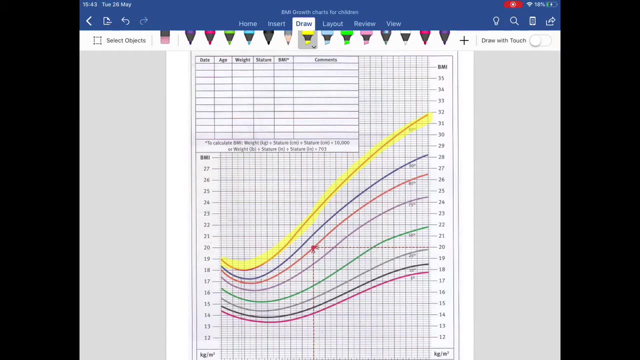 So this growth chart is for girls age two to 20.. If we look at our growth chart, You can see- we've seen this before and these colored lines are all the percentiles. So we have eight curves and those are eight percentiles. 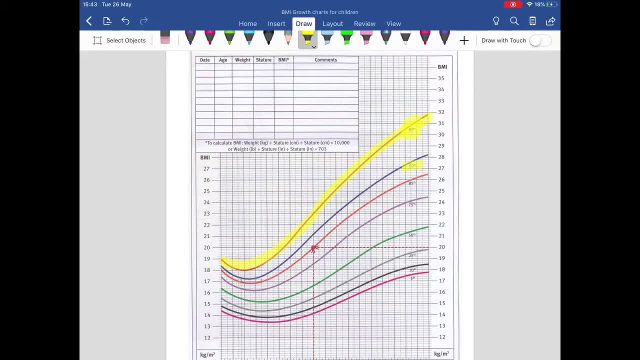 This one is the nihilist 95th percentile, the 90th, 85,, 75,, 50,, 25,, 10, and 5.. So, if you remember, 50% is average. So when we deal with statistics, 50% is the average and that is the average percentile. 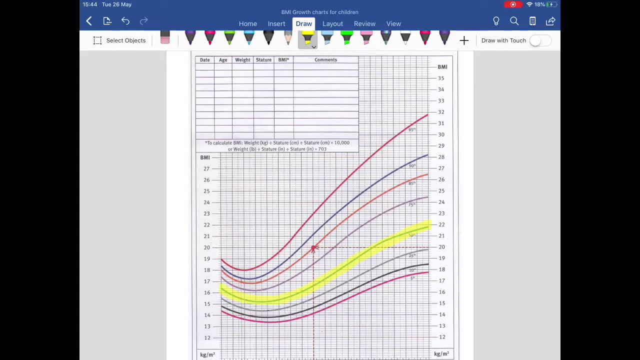 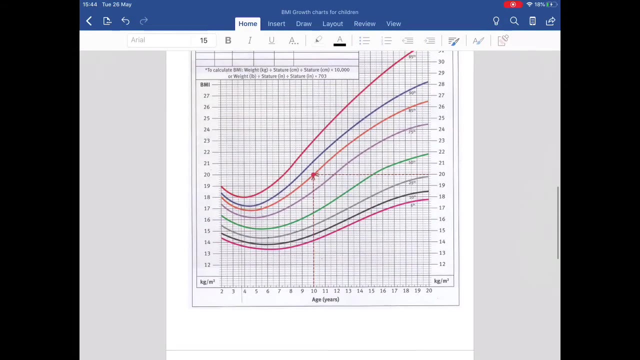 Okay. so let's have a look at what has been given to us here, and you will see that in the diagram they have marked this red dot over here. Now, what is that? Well, they are saying a 10-year-old. 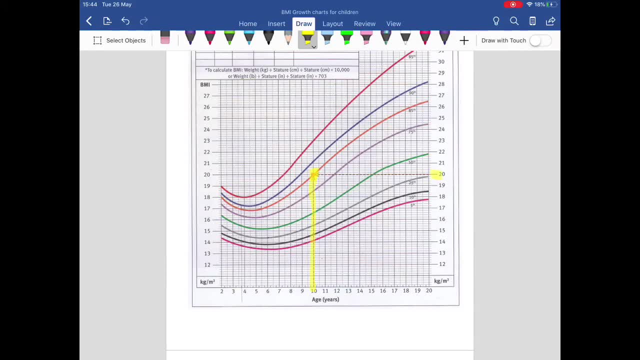 with a BMI of 10,. 20 is on the 85th percentile. So let's just have a look at it without the highlighted lines. So this child is 10 years old. This girl is 10 years old. She has a BMI of 20.. 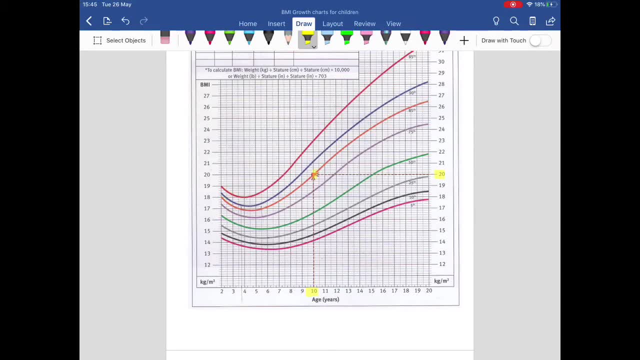 So we have to draw the two lines and where they meet, that is the percentile that she is on. So we have to draw the two lines and where they meet, that is the percentile that she is on. So she's on the 85th percentile, which means 85% of 10-year-olds with a 20 BMI are the same as her. 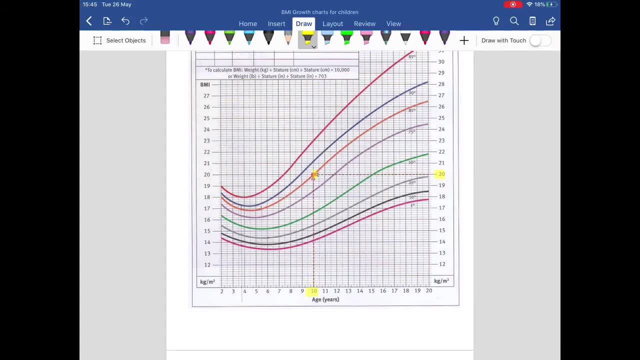 It also means that there are. so if this is on the 85th percentile, it means that 85% of girls 10 years old have a low BMI, have a lower BMI than what she does, And it also means that 15% of the girls that are 10 years old have a BMI greater than hers or higher than hers. 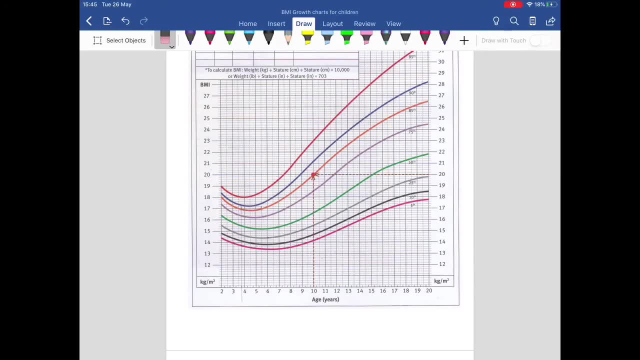 So is she average? No, In fact, she is above average because your average BMI is here. So the average 10-year-old should have a BMI of 20.. So the average 10-year-old should have a BMI of 20.. 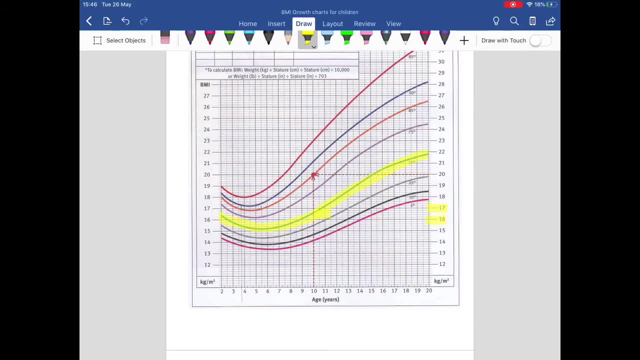 So the average 10-year-old should have a BMI of 20.. Now we can start adding more numbering. Now we can start adding more numbering. Now that we're looking at that, I want you to have a look at the scale on the side. 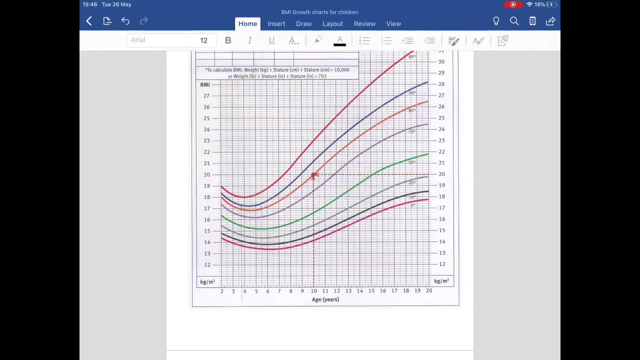 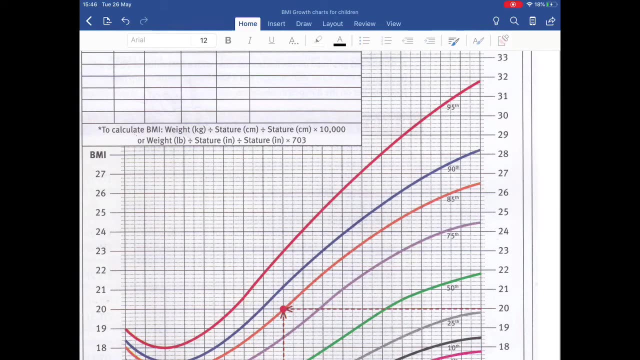 Remember, before you can read any graph, you have to be able to understand the scale. Now that we're looking at that, I want you to have a look at the scale on the side, So it doesn't matter where we are on the graph. 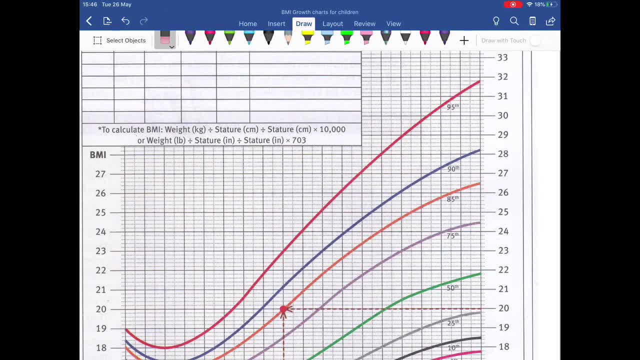 So let's take from 20 to 21 over here, So 20 to 21, this interval, So 20 to 21, this interval, And we can see. if I go and count these divisions, I've got 1,, 2,, 3,, 4, 5.. 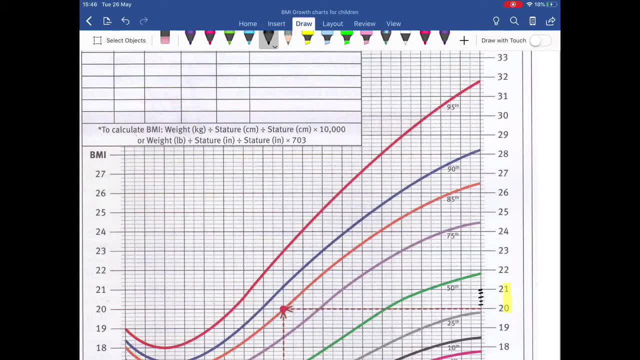 So I've got five divisions, which means one BMI unit is divided into five. So if I take one divided by five, I'm going to get 0, 2, which means this is 200 or 0.2.. So I would have. so the first one would be 20, 2,, 20, 4, 20, 6,, 20, 8, and then 21.. 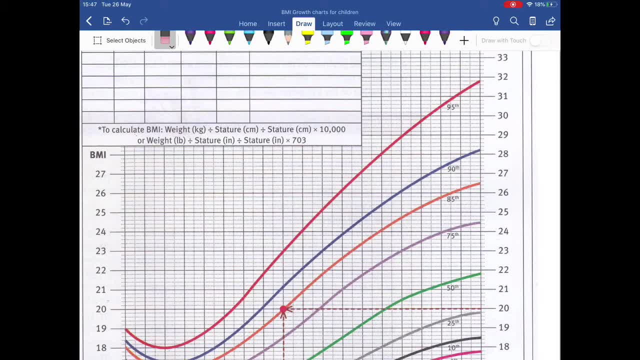 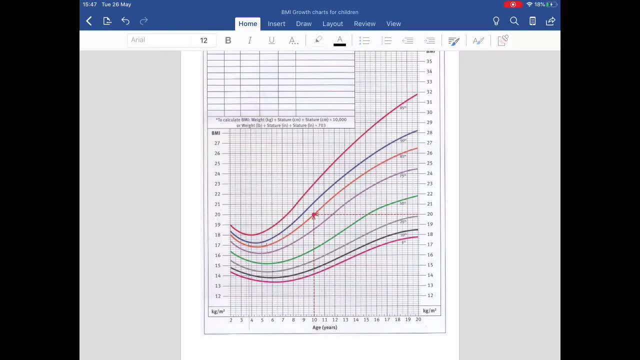 So that is how you work out the scale. Let's go back and look at a few more questions. Right, If I have a BMI Of 25.. So this person has a BMI of 25, this girl and is on the 90th percentile. 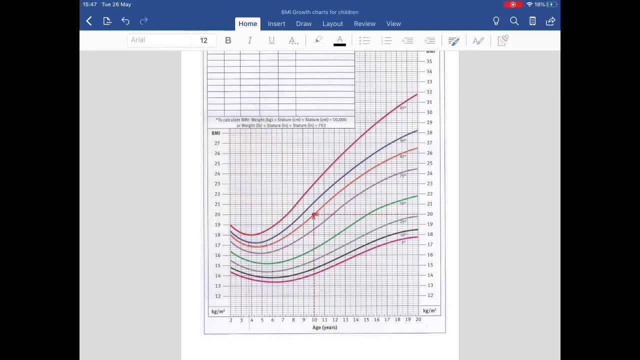 How old is she? Okay, So the BMI is 25.. So I will go along this line. You are then told that this girl is on the 90th percentile, which is the blue mark, and where those two meet, So 25.. 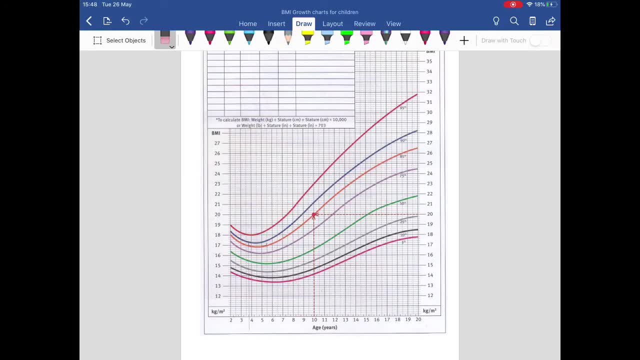 And 90. Let me just rub this out a bit So now we can see better. So 25 and the 90th percentile is there. I would then drop a line straight down, And it is in between, in the middle of 14 and 15.. 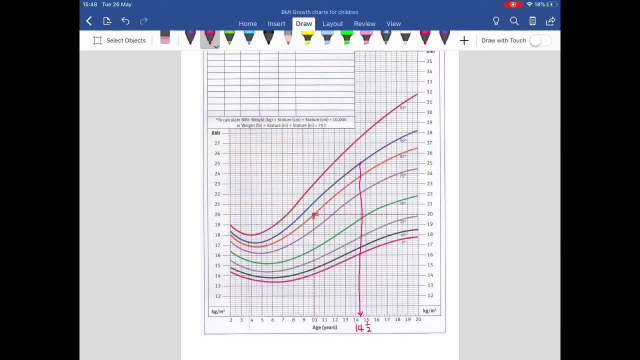 So this girl is 14 and a half years old. Her BMI is greater than average, So This child is probably overweight. I could also ask you: what would the average nine-year-old, what would the average nine-year-old's BMI be?